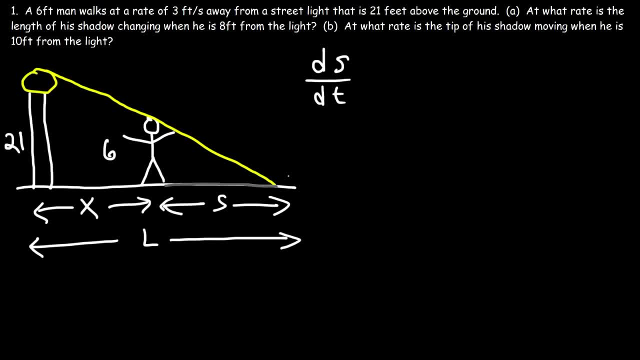 That's the rate at which the length of the shadow is changing. So that's how fast S is changing. Part B: at what rate is the tip of the shadow moving? when the tip of the shadow moves? In this case, that's going to be equal to the rate at which L is changing. 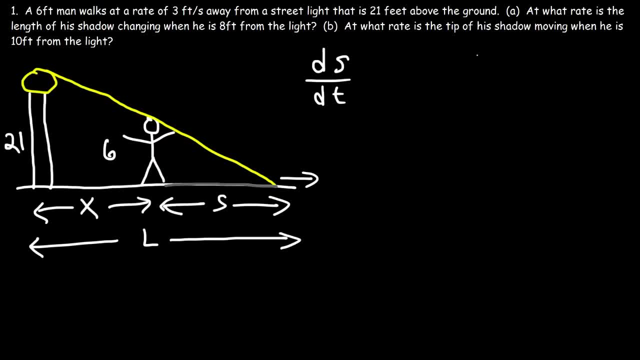 So part B is really looking for dsdt. So make sure you understand that. So dsdt tells you the rate at which the length of the shadow is changing, But dsdt tells you the rate at which the tip of the shadow is moving. 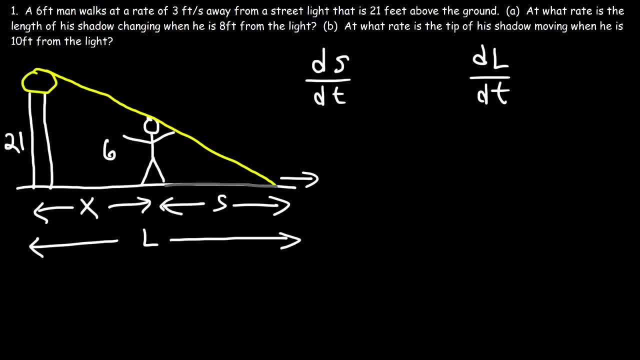 So how can we calculate dsdt? Let's start with that one first. What do we need to do in order to find it? Now, for this problem, you need to draw similar triangles, So let's draw the first triangle, That's the large one. 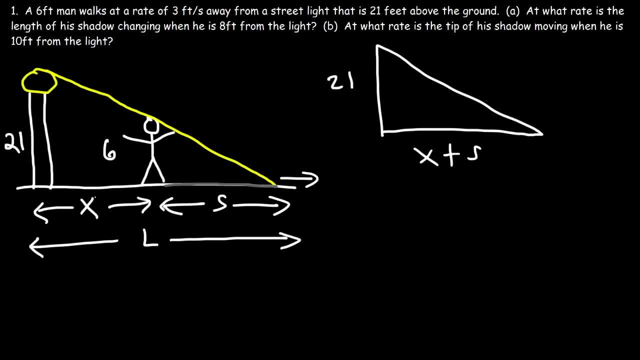 Where this is 21 and this is x plus s. So that's for this triangle right here. Now let's draw the second triangle, The smaller one, Where this is 6 and this is s. Now we need to set up a proportion between these two triangles. 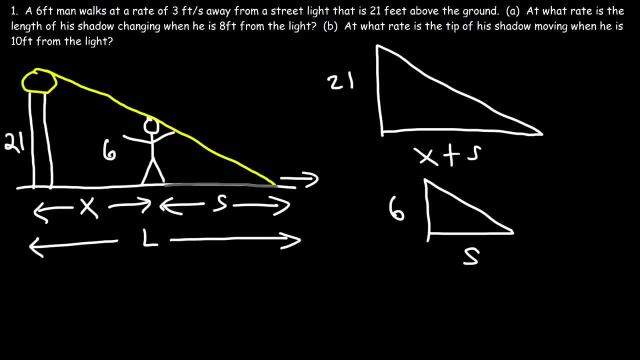 And if you're unsure how to do it, here's something that can help you to do it correctly. Note that these two triangles have the same angle theta. If you draw the large triangle, it has the angle theta, And the small triangle has the same angle theta. 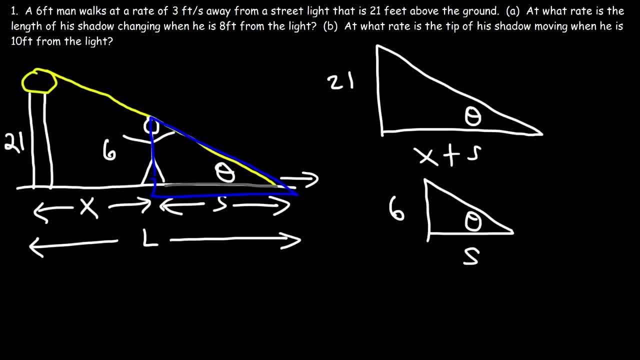 And both triangles are right triangles. Now, according to Sokotoa- hopefully you know your trick- Tangent theta of the first triangle, that is this one: it's equal to the opposite side, which is 21, divided by x plus s. 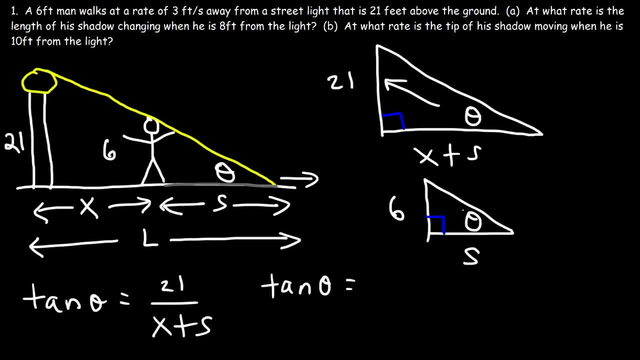 Now tangent theta of the second triangle. it's also equal to opposite over adjacent. So therefore we could set 21 over x plus 6, I mean x plus s- and set that equal to 6 over s. So we have this so far. 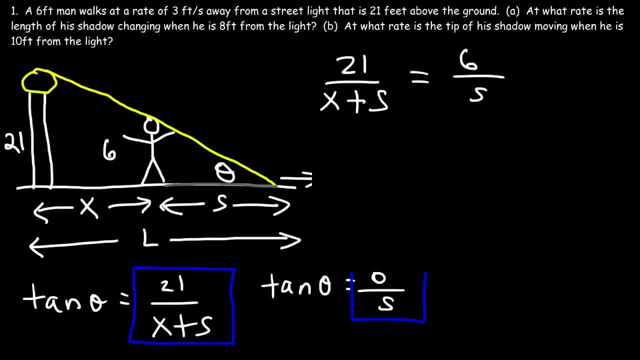 Whenever you have two fractions separated by an equal sign, you can cross multiply. So if we cross multiply, we're going to have 21s is equal to 6 times x plus s. Now let's distribute 6.. So this is going to be 6x plus 6s. 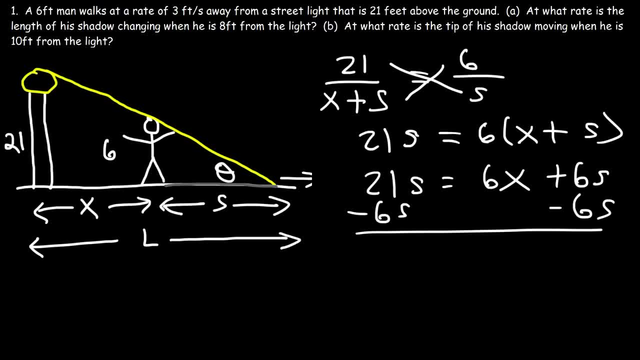 Next, we can subtract both sides by 6s. So 21 minus 6 is 15.. So we have 15s is equal to 6x. Now, once you get to this part of the equation, we can perform implicit differentiation. 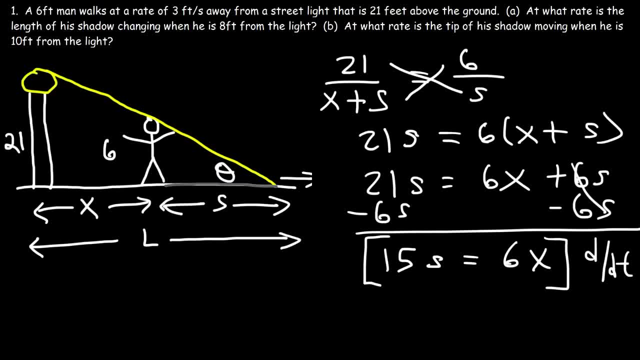 Let's find the derivative of both sides of the equation with respect to time. So the derivative of 15s is going to be 15 times the derivative of s, which is 1 times ds, e, t, based on the constant multiple rule. 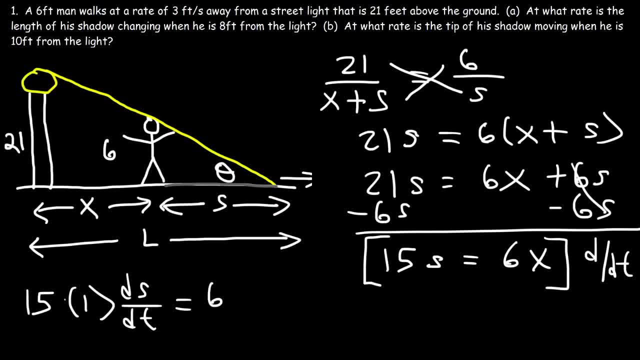 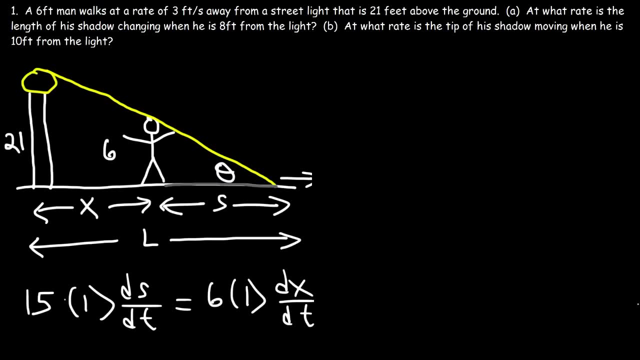 And the derivative of 6x is going to be 6 times, 1 times dx e t. So now, at this point, we need to plug in what we have. Our goal is to calculate ds e t, but we need dx e t. 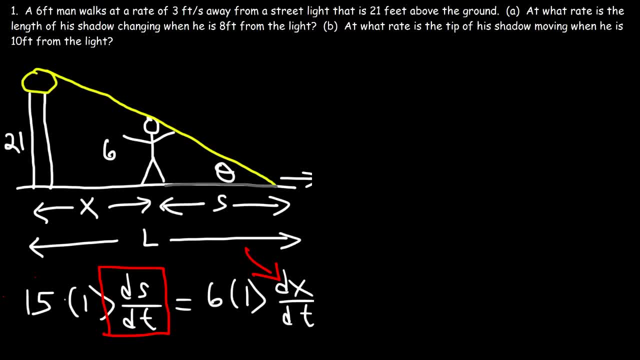 So what is dx e t in this problem? So notice that the man, he's walking at a rate of 3 feet per second away from the lamp, So he's going in this direction. Now that tells us the rate at which x is changing. 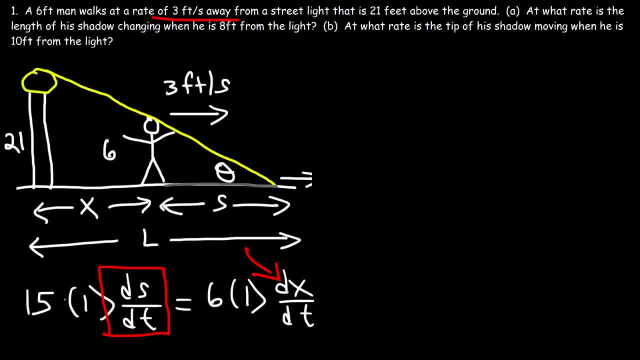 Every second x is increasing by 3 feet. So because x is increasing and not decreasing. if he was walking towards the lamp, x would be decreasing, But in this problem he's moving away from the street light, So x is going up. 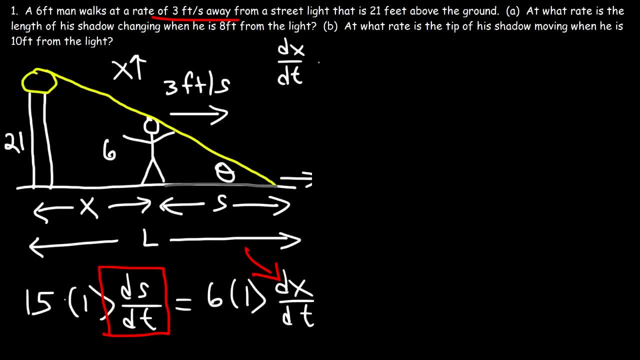 Therefore dx e t is positive 3 feet per second. If he was moving toward the street light, x would be decreasing and dx e t would be negative 3 feet per second. So now that we have dx e t, we can plug it into this equation. 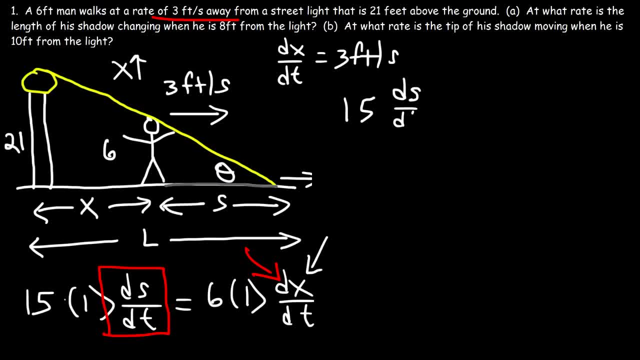 So we have 15 ds e t. that's equal to 6 times 3.. Now let's divide both sides by 15.. So ds e t is 6 times 3, and 15 is 5 times 3.. So we could cancel a 3.. 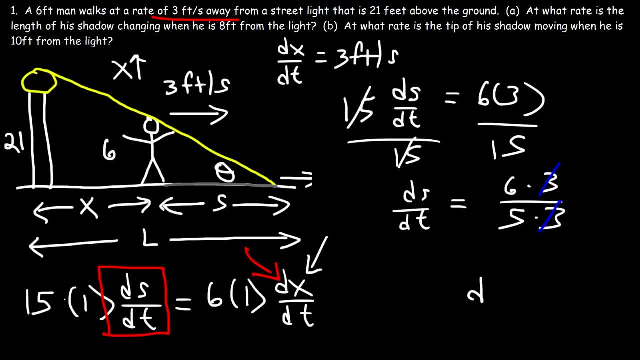 And now this gives us the final answer for Part A, ds, e, t is going to be 6 over 5 feet per second. So that's the rate at which the length of the shadow is changing. Every second it changes by 6 over 5 feet or 1.2 feet. 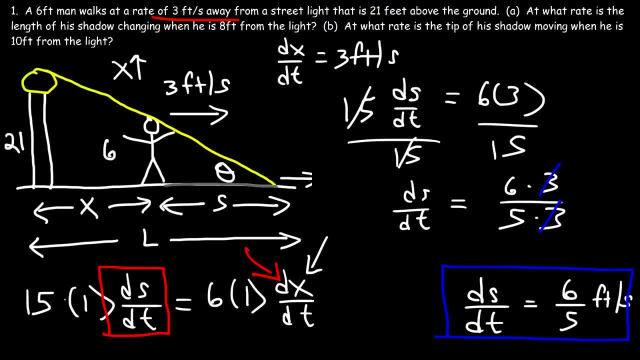 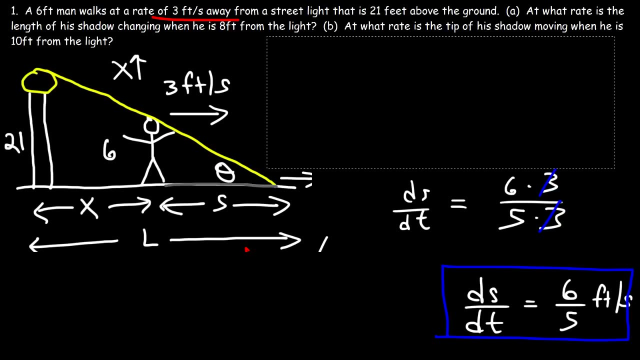 Now let's move on to Part B. At what rate is the tip of his shadow moving when he is 10 feet from the light? So this time we need to calculate d, l, d, t. How can we do that? First, let's get rid of some stuff. 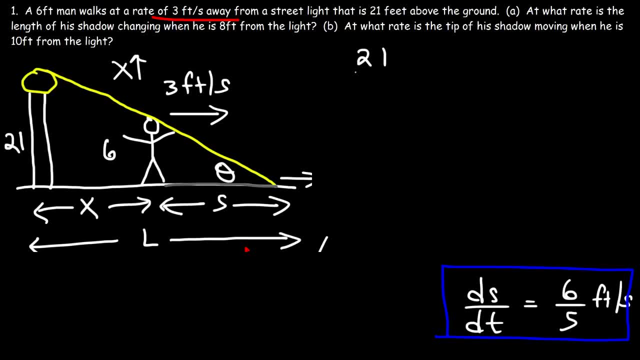 Now let's start with this equation which we had earlier: 21 divided by x plus s is equal to 6 over s using similar triangles. Now, instead of using x plus s, we're going to replace that with l, Because notice that x plus s is equal to l. 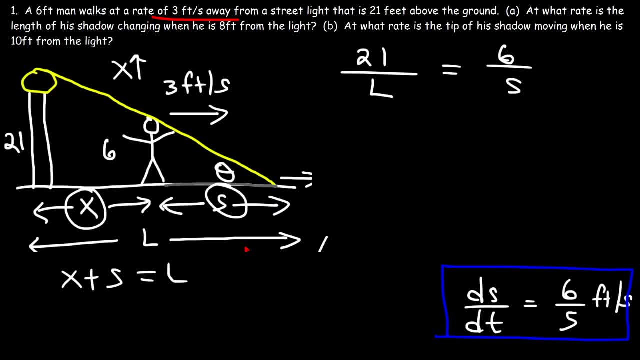 So therefore we have this expression: 21 over l is 6 divided by s. Now let's cross, multiply, So we have: 21s is equal to 6 times l. And now, in this form, let's differentiate both sides with respect to time.